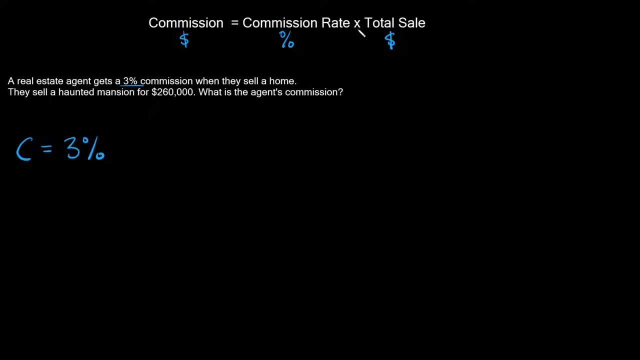 So I'm going to put three percent and then we're going to multiply that by the total sale, right? What was the total sale? It was two hundred sixty thousand, right? So times two hundred sixty thousand dollars, All right, how am I going to? 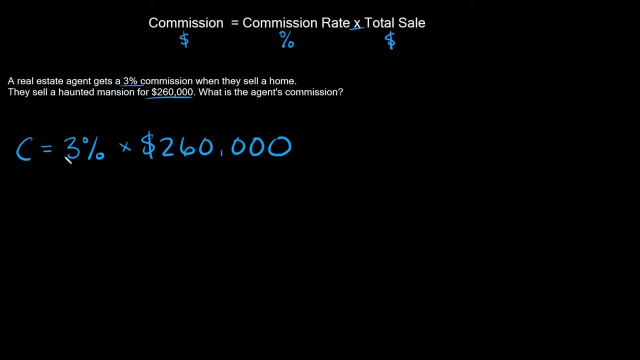 solve this? Well, the first thing you have to do is turn this percent into a decimal. okay, You can never have a percent in one of your formulas. You always have to convert it to a decimal first. okay, So your commission is going to be equal to. now. let's write three percent as a decimal. How? 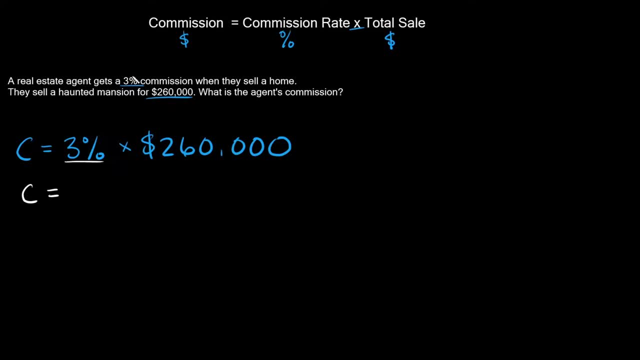 would you do that? Well, I'll do it up here, and the easy way of doing it is just drop your percent symbol, okay. So what number do we have here? We have the number three, right? Okay, where's the decimal on the number three? It would be. 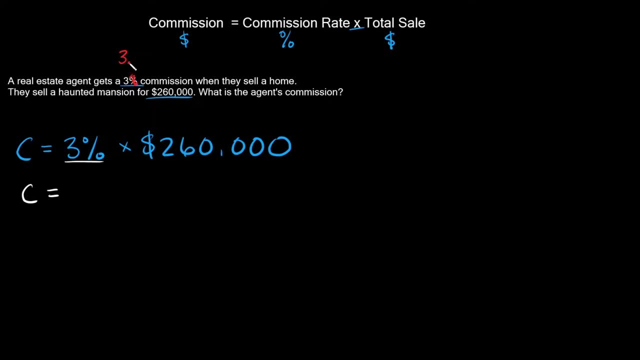 right there, right? So all you have to do is grab your decimal and move it two times to the left. So we're going to go one, two, okay. So that's where your decimal is now And, as you can see, we have. 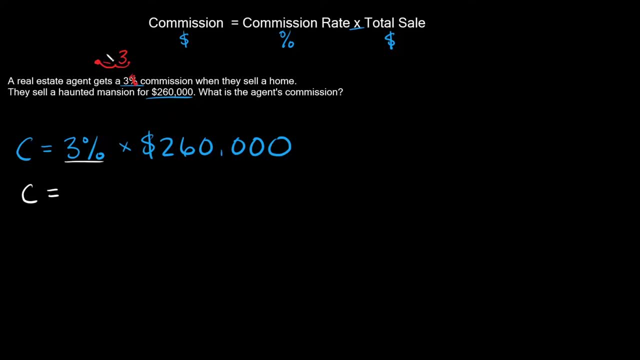 an empty place value right here. So whenever you have an empty place value like that, in order to fill in the blank, you just put a zero right there, okay? So three percent as a decimal would be point zero three, okay, So I'll write that right here: point zero three, okay, And the more proper. 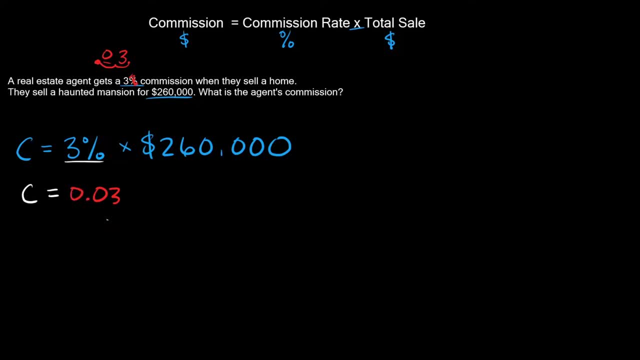 way of writing this decimal would just be putting a zero right there as a placeholder right. So zero point zero three, And then we're going to multiply that by 260,000.. 260,000.. Okay, so now you just have to throw this into your calculator. 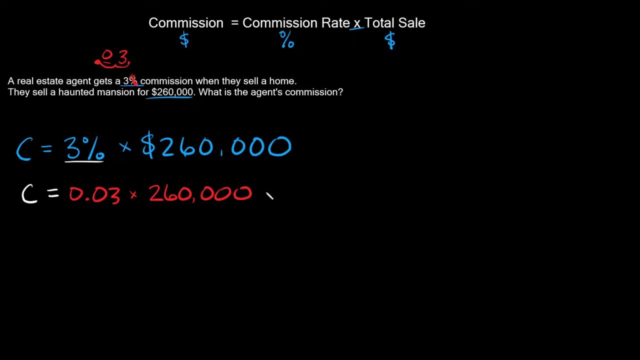 Point zero, three times 260,000 is equal to 7,800.. So your commission is equal to 7,800.. 7,800? what? Well? remember, the units for commission are dollars, right? So I'll put a dollar sign, right. 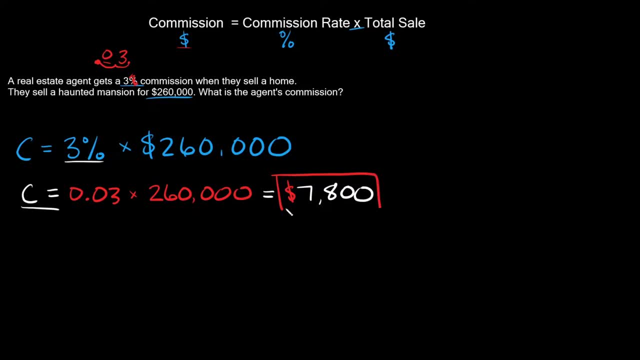 there. So the commission is equal to 7,800 dollars, right? Hopefully that wasn't too bad. Let's try one more example here. Okay, so this problem says a toilet salesman sells a fancy toilet that plays music and tells you funny puns about Winnie the Pooh- Nice, He gets a $69 commission. 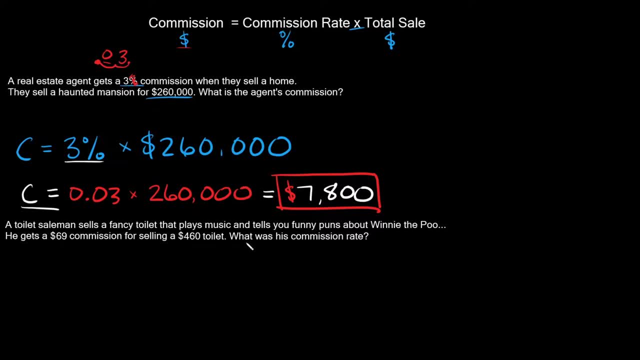 for selling a four-person toilet. So he gets a $69 commission for selling a four-person toilet. So he gets a $460 toilet. What was his commission rate? Okay, so this time we're not looking for the commission, We're looking for the commission rate, right? So how would we solve for that? 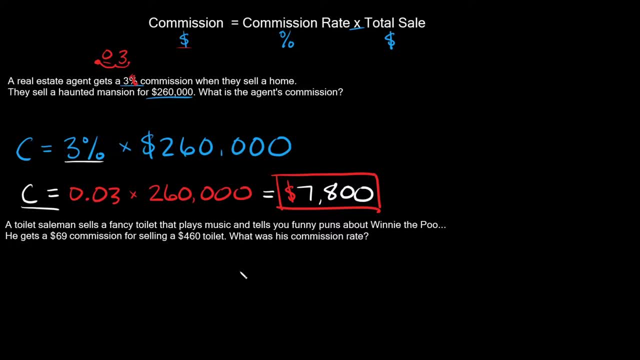 Well, let's just use our formula up here and just plug in what we know, okay? So we know he got a $69 commission, right. So his commission was $69.. So I'll put that right here. And that's going to be equal to right, Equal to his commission rate. 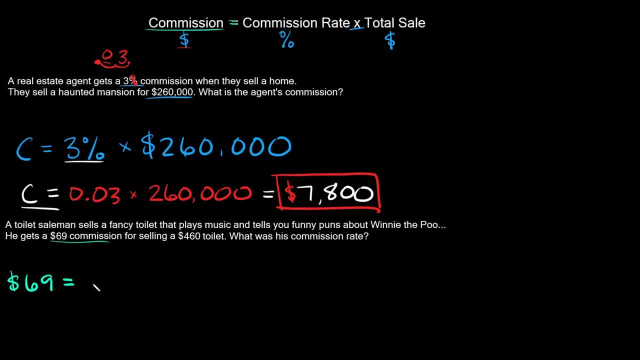 So that's the part we don't know. So I'll just put a variable there. for now I'll put R for rate And then we're going to multiply that by the total sale right. So we're going to multiply by however much he sold it for. So, selling a $460 toilet, So he sold it for $460.. 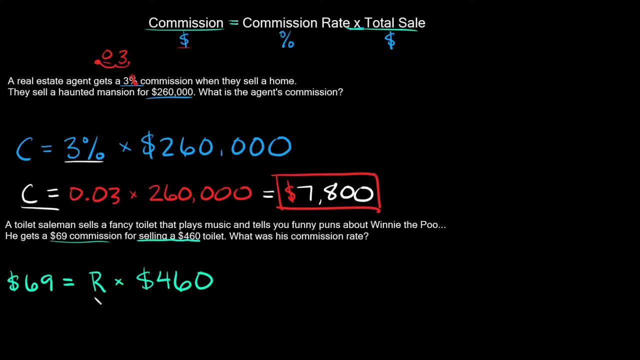 Okay. so here we have: $69 is equal to R times $460.. So how do we solve for R? right here? We want to isolate this variable by itself on one side of this equal sign, right here, okay. So in order to do that, or in order to undo the multiplication we're going to divide, okay. 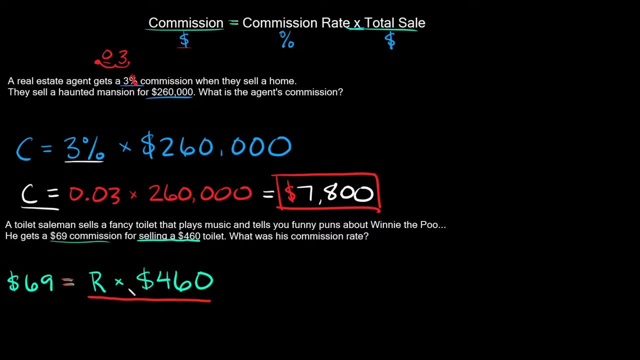 Divide by what? Well, whatever you're trying to get rid of. So if we want to get rid of the $460, we're going to divide by $460, okay. But whatever you do to one side of the equation, you have to do to the other right. So we have to divide by $460 on this side. 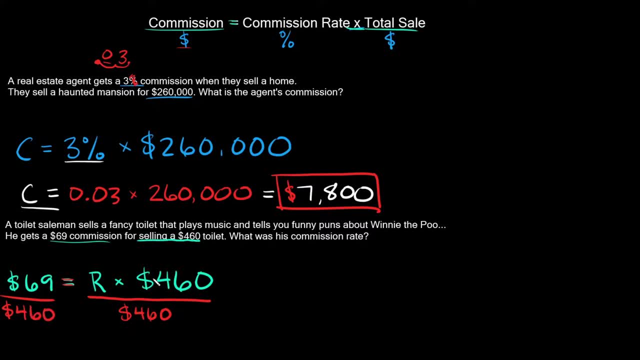 also. So we're going to divide by $460 on this side also. So we're going to divide by $460 on this side also. Okay, so now simplifying some things, These $460s. so there's one on top, one on the. 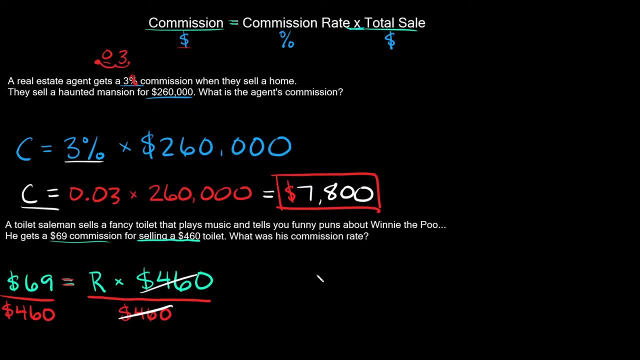 bottom. so those cancel out. So we're just going to be left with R right here on this side of the equation, okay, And then that's going to be equal to right, Equal to $69 over $460.. $69 over $460.. 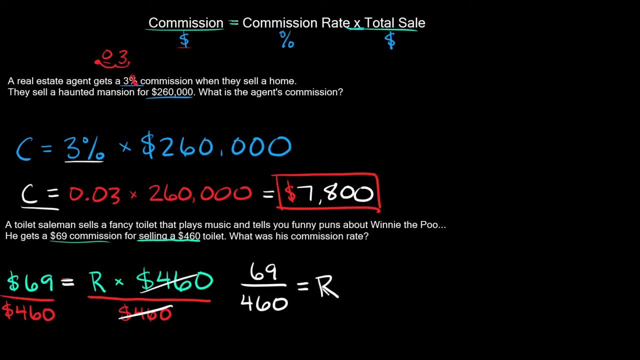 Okay, so now you just have to throw this into your calculator. So $69 divided by $460 is equal to 0.15.. And remember, that's equal to R. right, It's equal to R. So is this our answer, right here?